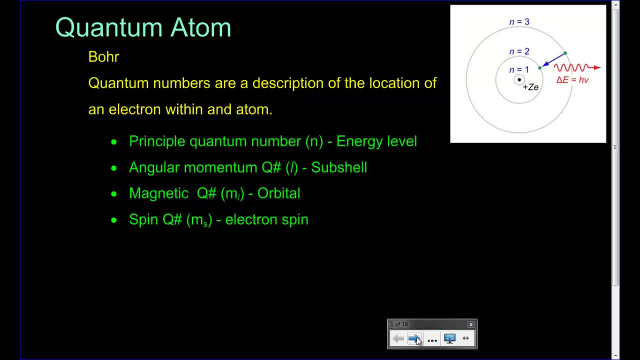 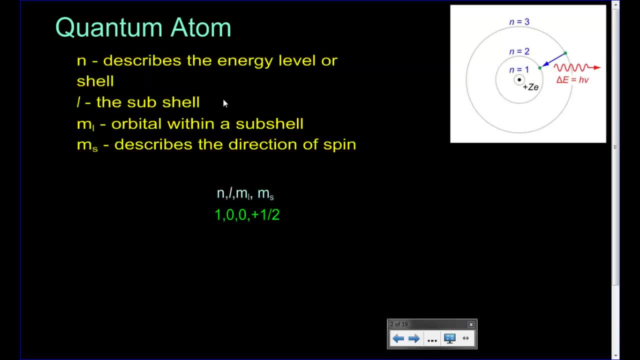 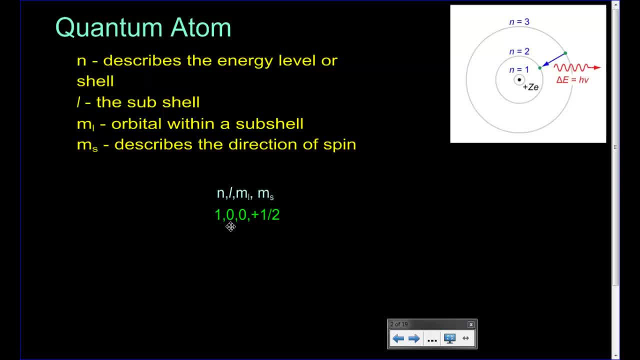 code for a location of an electron. And so when we get in here, first N, which is the level, It's in a zero subshell and that's just an indication. It's not telling us the quantity, It's just telling us a position. ML, so its orbital is the zero orbital and 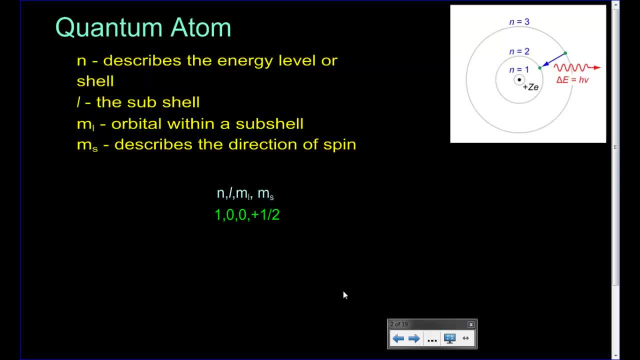 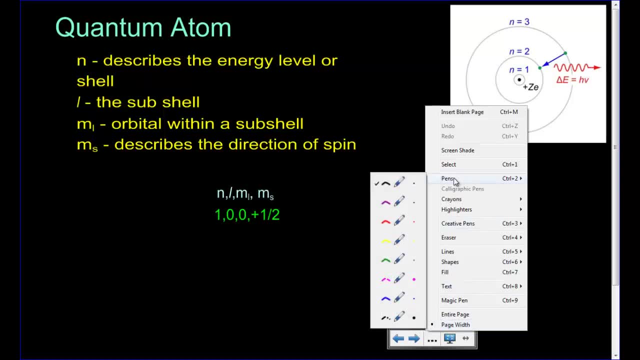 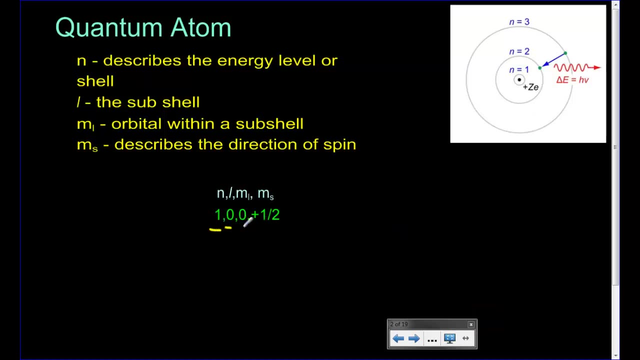 this electron is spinning with a plus one-half spin. So electrons can spin with positive or negative spins, and they're always one-half. So as we go down through this and start to look at this, so we have this first energy level, a zero subshell, a zero orbital and 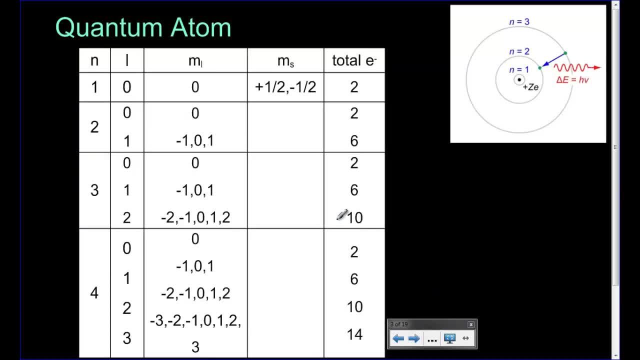 I'm spinning with a plus one-half spin. Okay, this is the description of quantum numbers. So if I'm in the first energy level, so that means that guy right there, there is one subshell and that's the zero subshell. I'm sorry, this is the zero subshell and 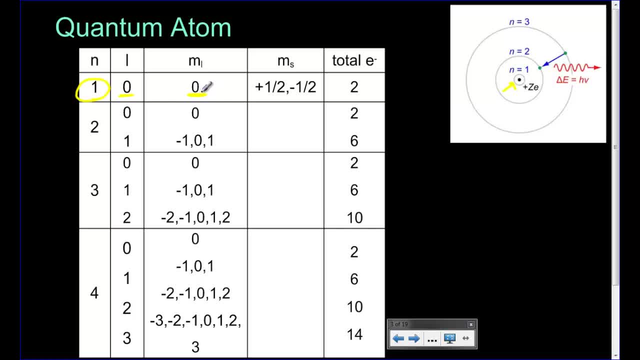 it has one orbital- It's called the zero orbital- and it has a possibility of a plus one half spin and a minus one half spin. So we have a total of two electrons that can exist there. Now we jump to the second energy level. We have two subshells. We call it the zero. 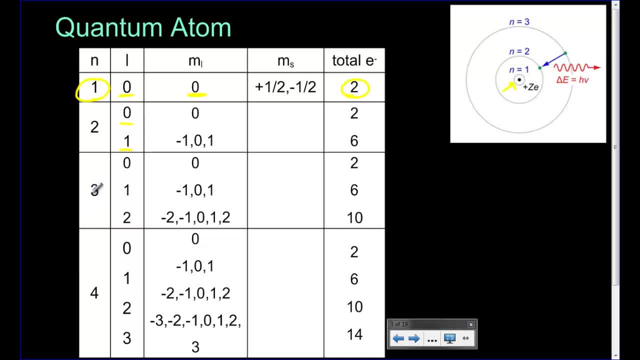 and the one subshell. So if you notice, as we go down to each energy level, each n value, that it always starts with a zero. So the subshells always start with this simplest subshell. and in a zero subshell you have one orbital called the zero orbital. In a 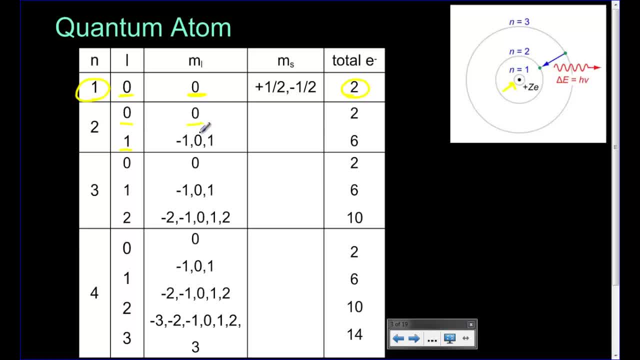 one subshell. you have a minus one half spin and a minus one half spin, So we have a total of three orbitals. One of them is called negative, one zero and one, And in each of those you have each one of these orbitals, you have a plus one half minus one half. This would 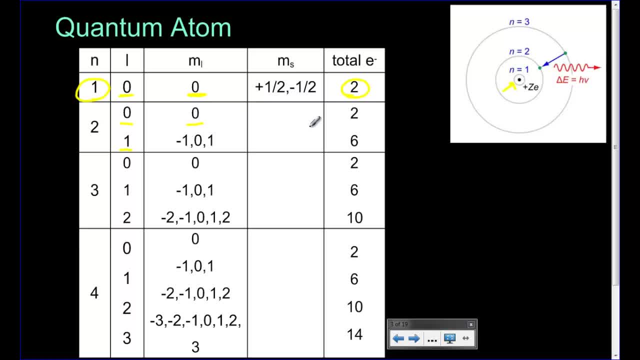 have a plus one half minus one half, plus one half minus one half, and so on. So you notice that if you have one orbital you have two electrons, If you have three orbitals you have six electrons, And you'll notice that pattern kind of continues down And so 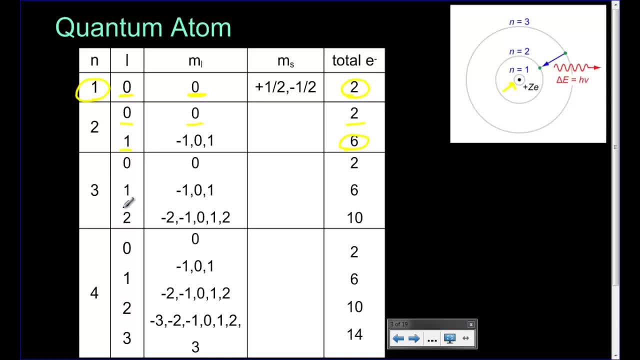 L is always zero to one, So you'll notice that L is always zero to one, So you'll notice that you'll notice that one less than the energy level. And then the orbitals are always from negative, whatever the subshell is, to positive, In other words, if this is one. 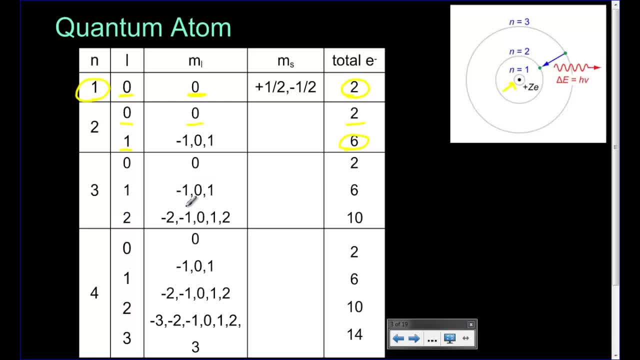 then it's negative one, zero one. If it's two, it's negative two, negative one, zero one, two. And if you notice, we have one orbital, we have three orbitals, So six electrons, And now we have five orbitals and so we get a total of ten electrons. And so you'll notice, 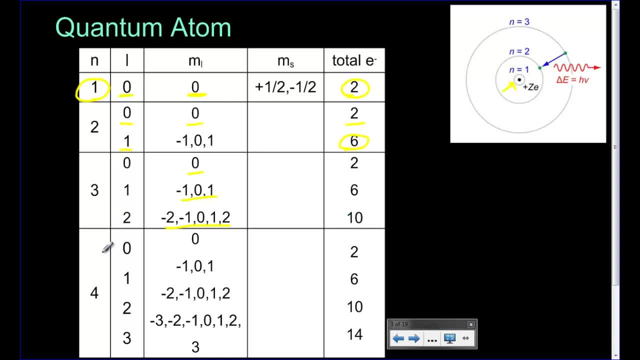 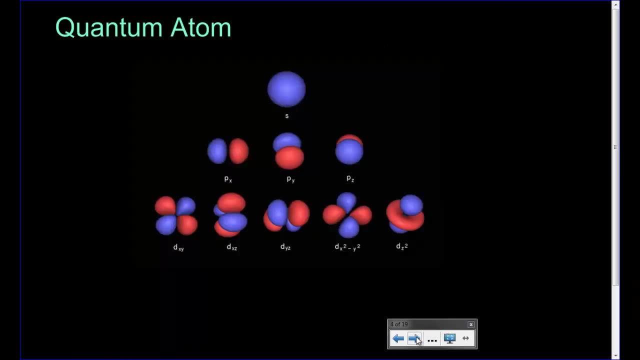 Bohr came up with this idea of quantizing or giving a description for the location of an electron, And what we're going to do is- you guys will experiment with this a little more- but what it leads to is understanding what those orbitals start to look like. 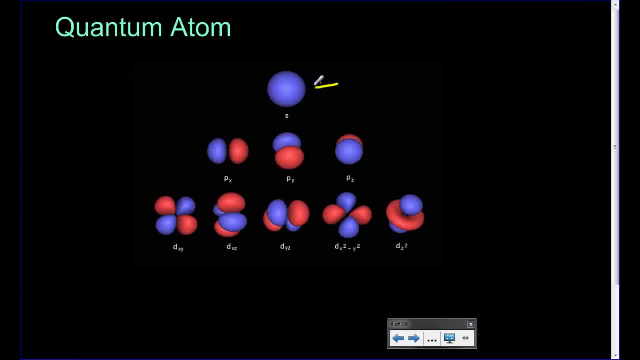 And so a zero orbital. if we look at this first thing, these are zero orbitals, Whether they're a 1-0 orbital, a 2-0 orbital, a 3-0 orbital. in other words, n is 1,, 2, or 3,, but the l value is 0,, 0,, 0, okay. 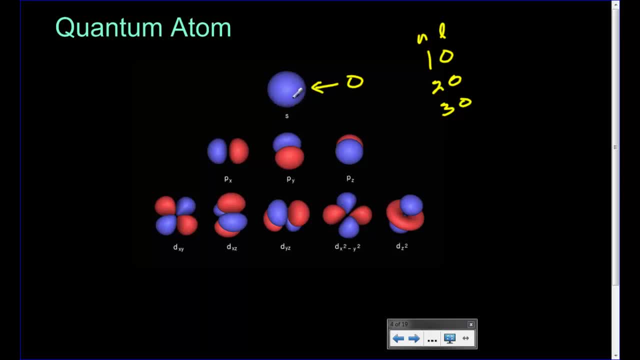 So that is a zero subshell and also a zero orbital, So we could do this: 0, 0, 0.. Okay, so that describes what's going on with an s, And so when we see this arrangement, that actually indicates, for our sake, 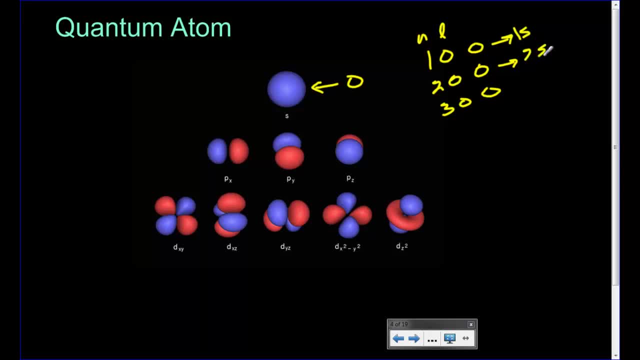 we're going to say that's a 1s, and this is a 2s, And this guy would be a 3s. And now, as we look down here, here's our p orbitals, which would indicate a minus 1,, a 0, and a 1.. 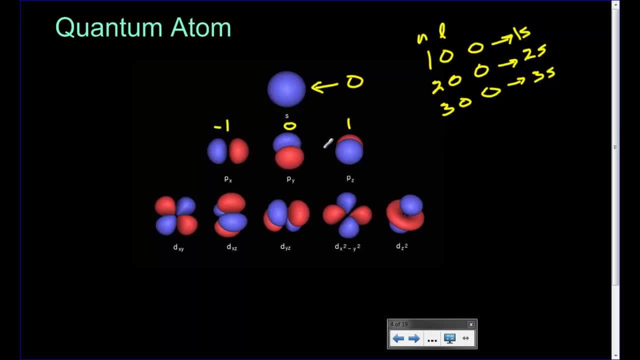 So here's what we have is in the first energy level we don't have any p's, so we have to start in the second. So we go 2, 1.. 1 indicates that we have p subshells. 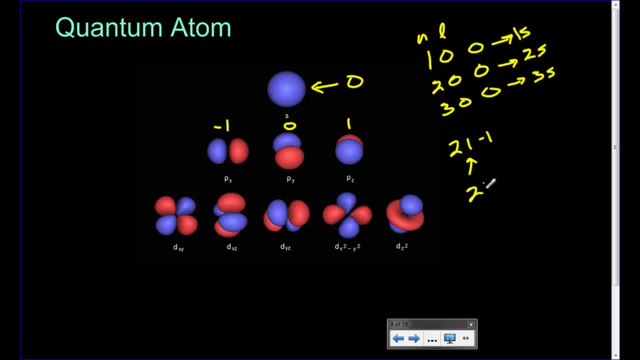 And you could say negative 1.. You'd go 2, 1, 0.. 2, 1, 1.. So those are the quantum numbers, for this would be 2p, and actually we could say 2p- 1,. 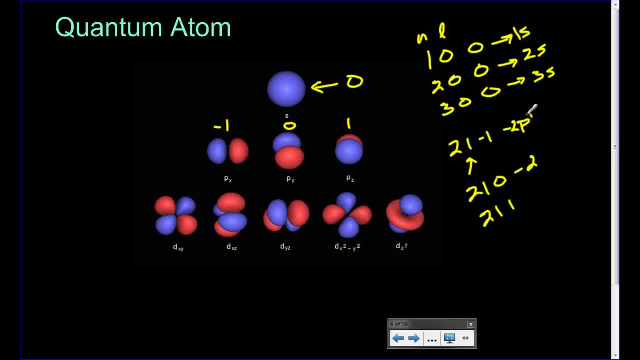 because there's one electron, and then we could actually have two electrons there And so we could say 2p and there's two electrons in here, so we have a total of a possibility of 2p, 4. And here we could have actually 2p. 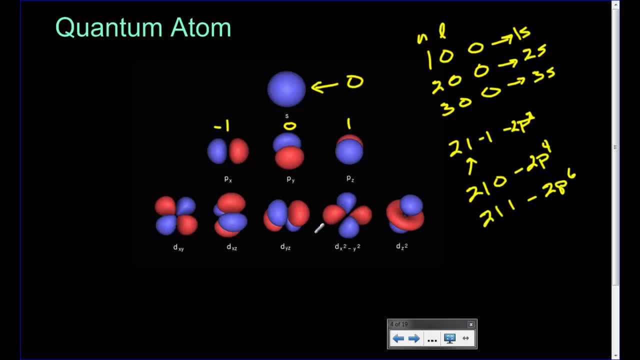 2p, 6. And so a total of those six electrons. Down here we have the d's, and this would be minus 2, minus 1,, 0,, 1, and 2.. So that indicates those orbital shapes based on these quantum numbers that we've talked about. 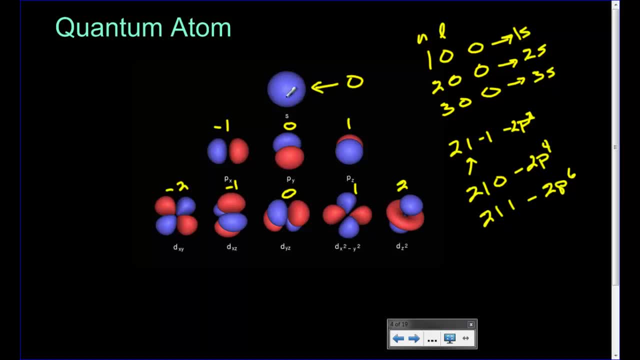 So when I start to talk about an s orbital, we're talking about this ball shape. When I start to talk about a p, there's these two regions where the electrons live. If I talk about d's, Only two electrons exist in here, but they can exist in any of those four lobes and so on. 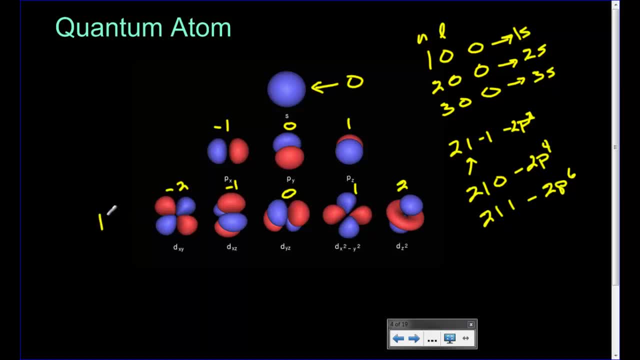 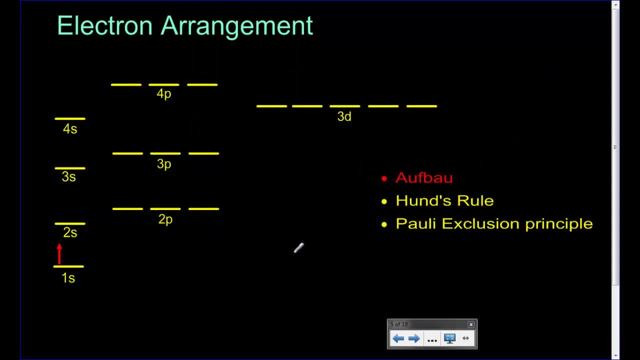 So if we look at the d's, we have five orbitals, so we have a possibility of ten electrons. Now, as we move on, when we start to look at these electrons, we kind of have to figure out. atoms start to build from the bottom up. 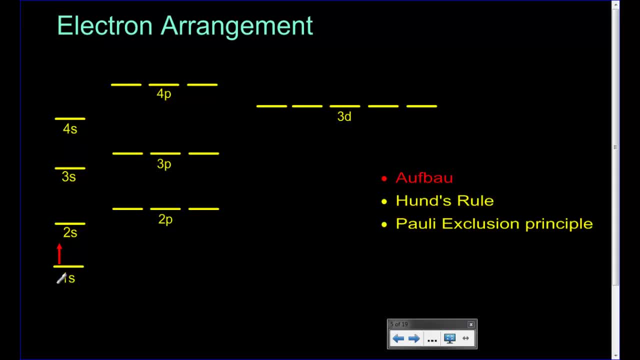 They start out at the very bottom, so they start at the 1s and they put one electron in there, And actually this could be hydrogen, because hydrogen tends to have. well, it has one proton and if we put one electron in, we have one electron orbiting around the outside of hydrogen. 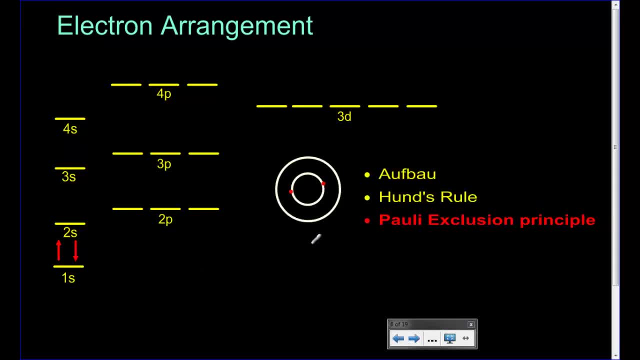 If we put a second electron, you'll notice we've filled up that first energy level, that s orbital, and we have two electrons. This would be, we could say, helium. And if we move on we go to three electrons and notice the next electron has to jump up into the 2s. 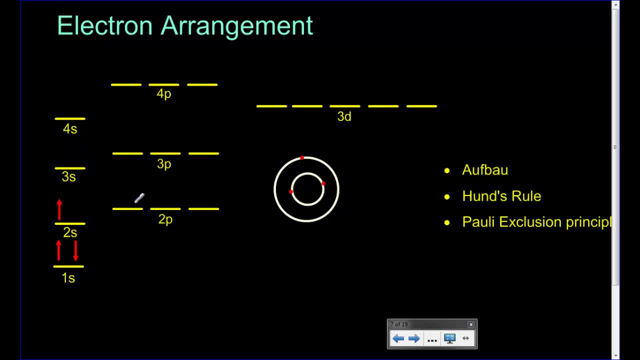 2s, orbital and subshell. And so what happens is we get this one electron out. in the next energy level We put another electron in there. Now notice that we have these arrows going opposite directions. This first arrow is that little plus one half, and the second energy is a minus one half.